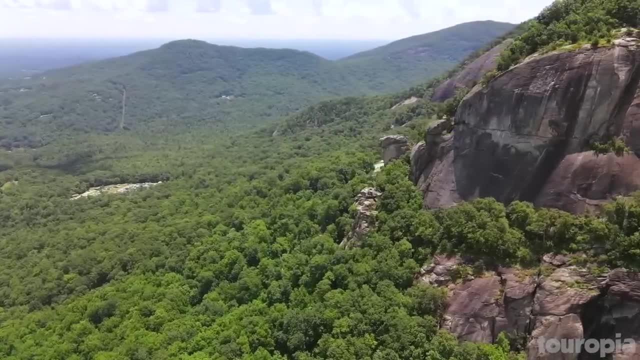 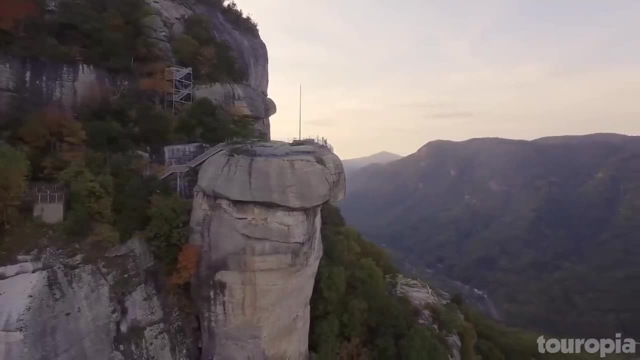 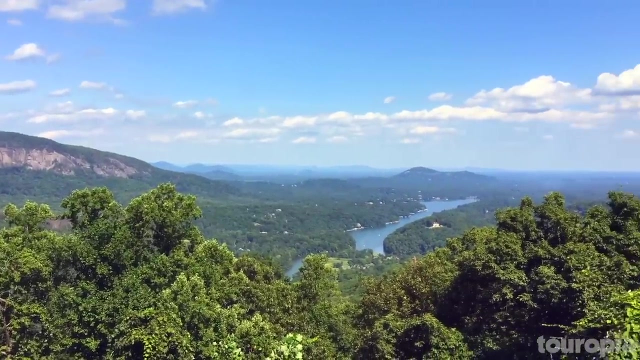 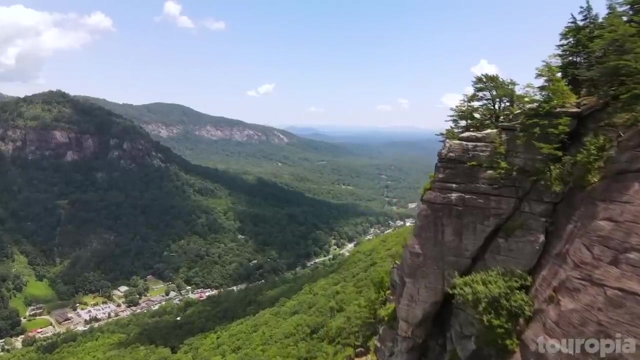 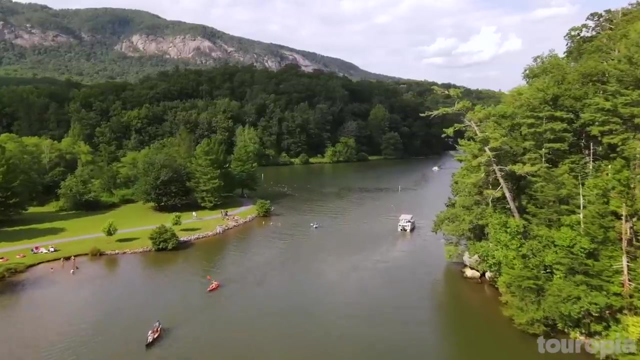 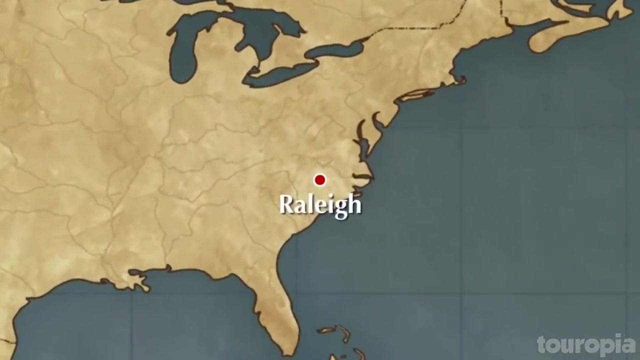 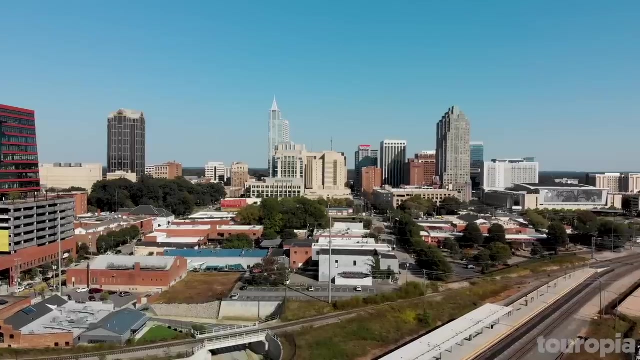 which boasts amazing views of surroundings. Visitors can either take the 26-story elevator or climb 500 steps to reach the top of the chimney Number 9. Raleigh: With a big city feel and plenty of southern charm, Raleigh continues to grow in stature and popularity. 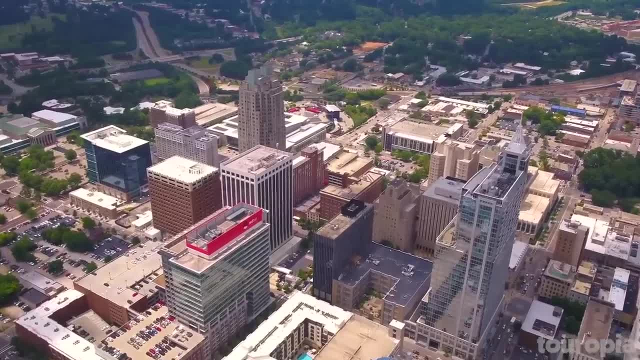 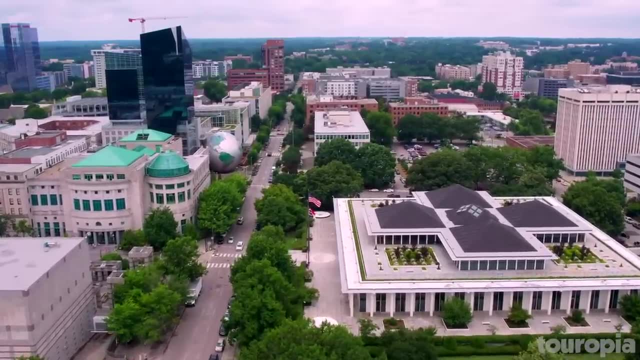 Visitors can make the most of the modern amenities while never being too far from nature. As the capital of North Carolina, Raleigh is home to some of the state's best museums and galleries, The cultural experiences, along with the sporting events and local markets within the downtown core. 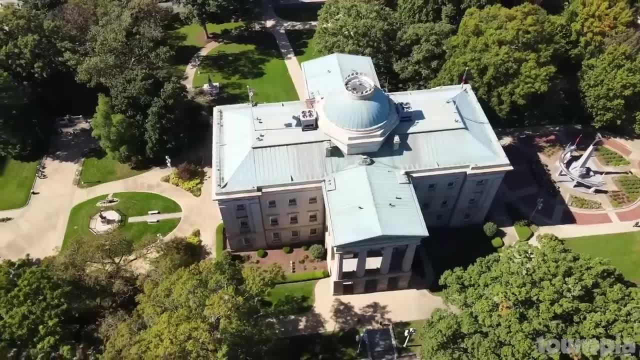 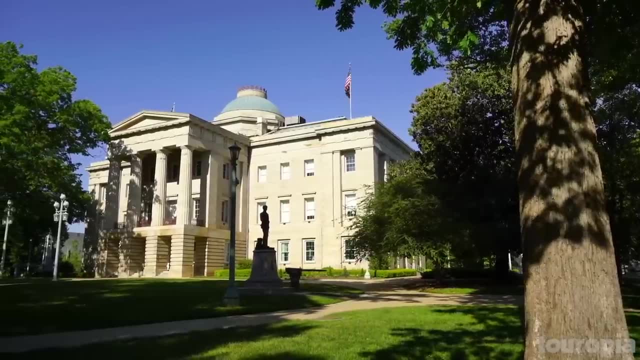 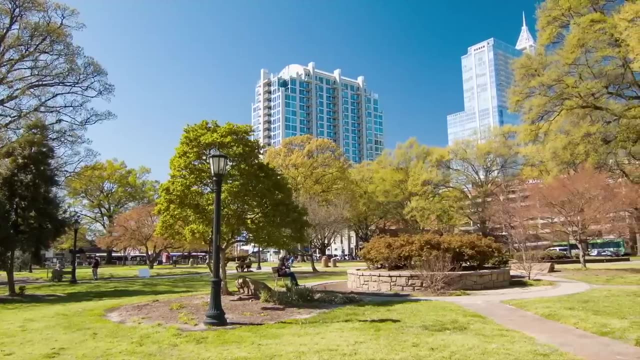 means there's plenty of things to do in Raleigh. However, Raleigh refuses to overgrow the surrounding natural area, leading to trails, parks and an abundance of outdoor adventures. The Chimney Rock State Park is home to the Chimney Rock Museum, a museum of the history of the Chimney Rock. 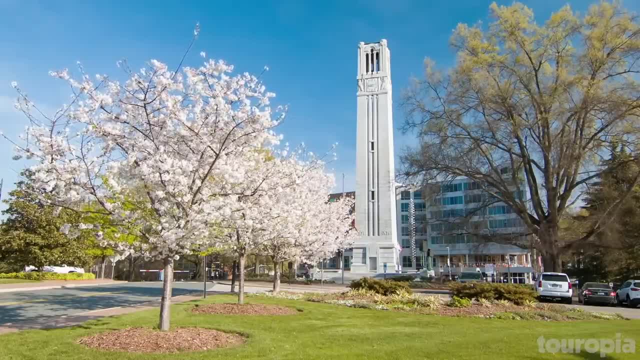 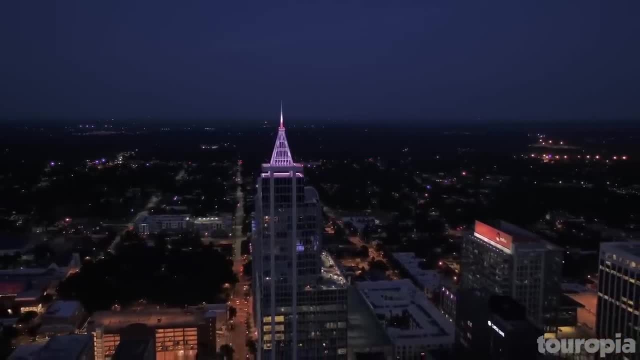 and the Chimney Rock Museum. The museum is also home to the Chimney Rock Museum, a museum of the Chimney Rock Museum, a museum of the Chimney Rock Museum, and the Chimney Rock Museum and the Chimney Rock Museum. 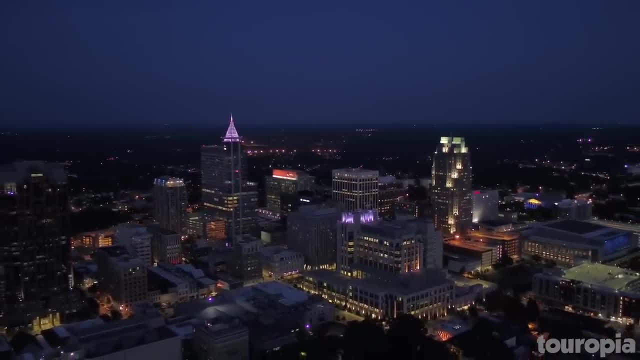 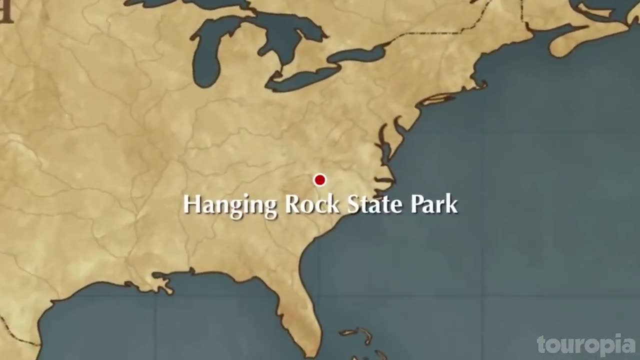 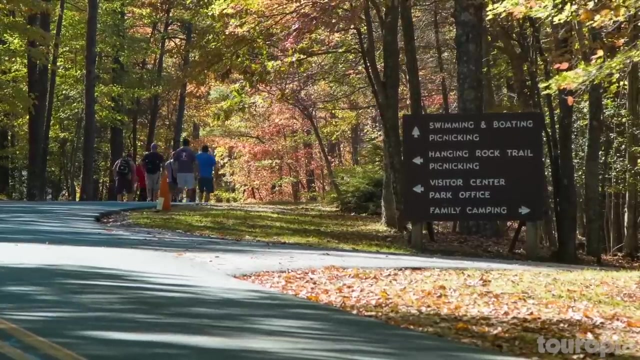 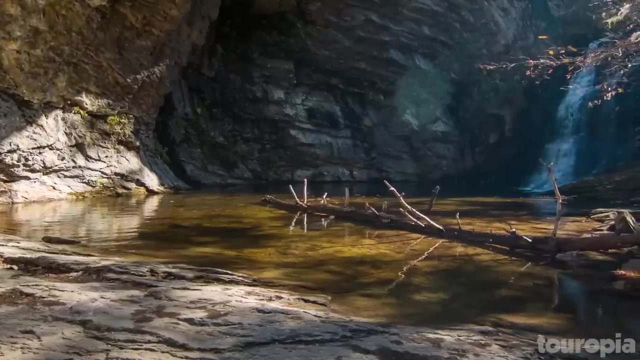 and the Chimney Rock Museum, Number 8.. Hanging Rock State Park. This lovely park, which is located close to the Winston-Salem area, offers visitors over 18 miles of trails that range from easy to difficult and a lake that is perfect for boating, fishing and swimming. 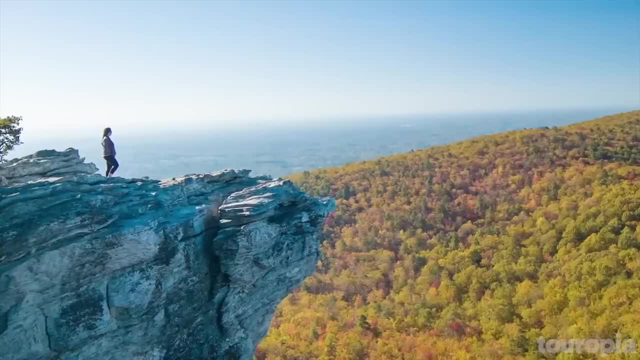 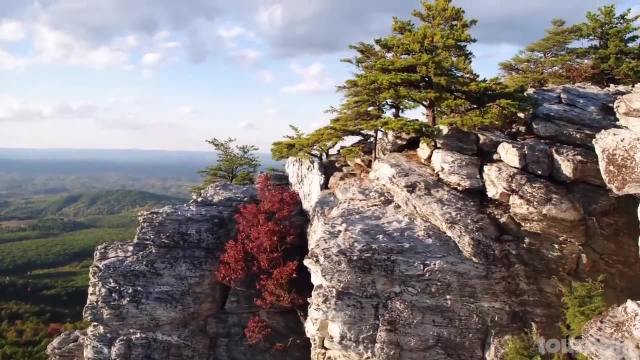 It is famous for its stunning quartzite formations. It is famous for its stunning quartzite formations and ridges, such as the Devil's Chimney and the eponymous Hanging Rock. The park is also home to a number of pretty falls. 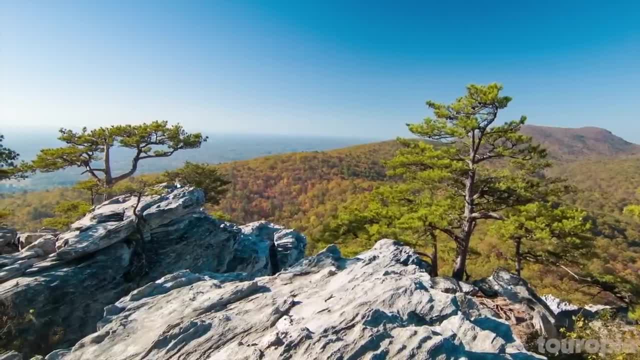 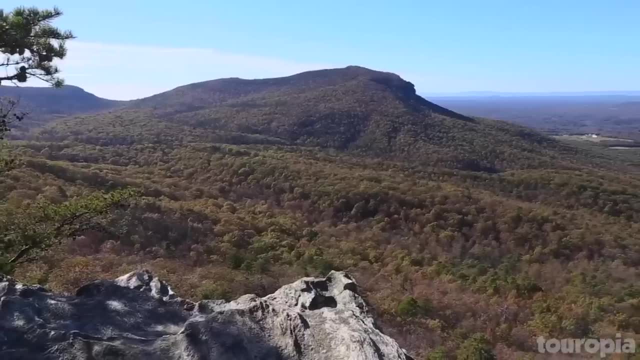 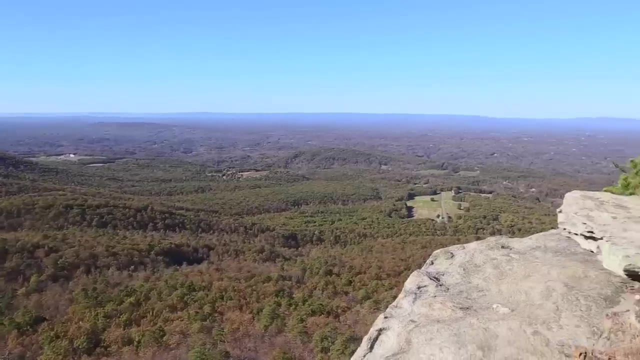 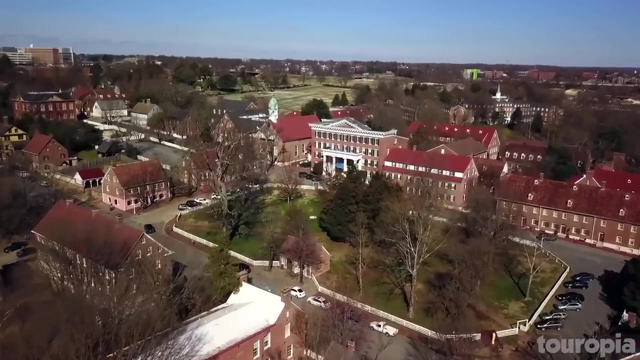 Hanging Rock State Park has 10 cabins, as well as a tent and trailer campground available for visitors who want to stay in the park. Number 7. Old Salem. Old Salem is a living museum, a recreation of what life was like in the Winston-Salem. 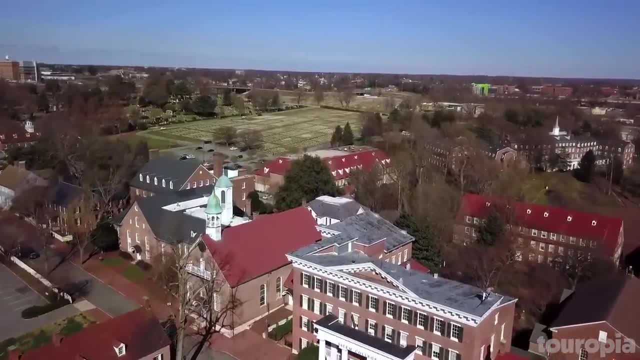 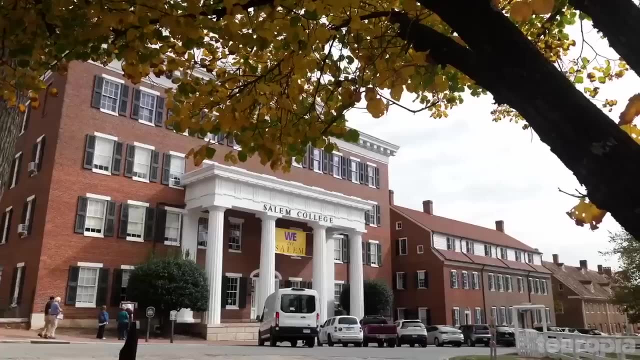 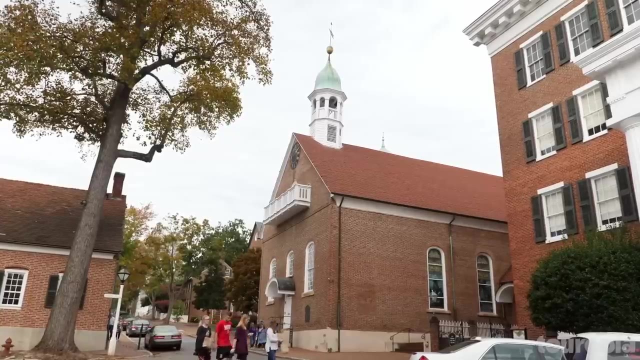 area of North Carolina during the 18th and 19th centuries. Through interactions with Old Salem's reenactors and by strolling the streets of this National Historic Landmark, visitors can see and experience firsthand the culture and various traits of the Moravian settlers who lived in this area. 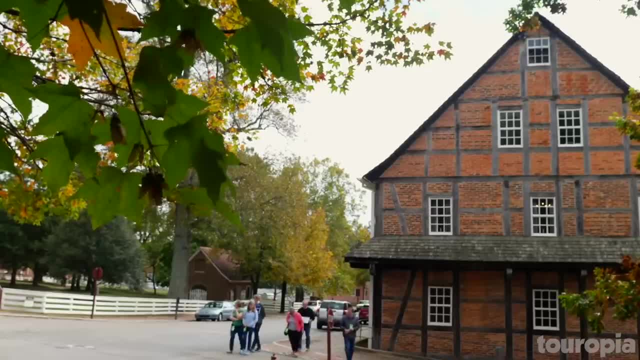 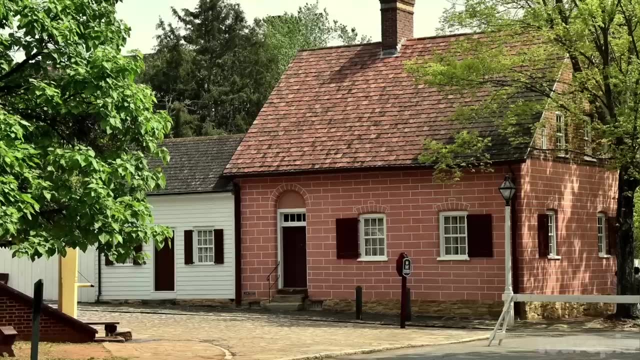 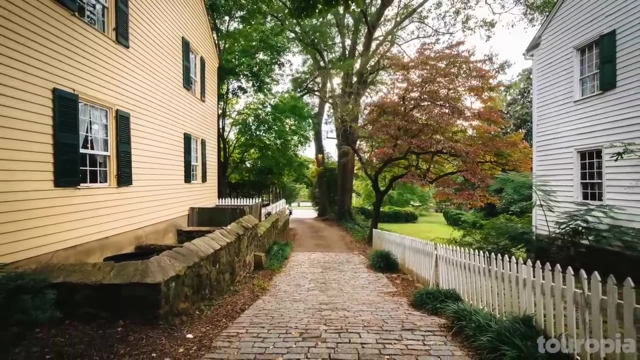 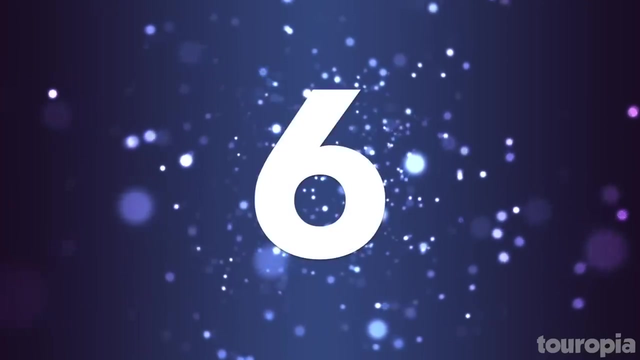 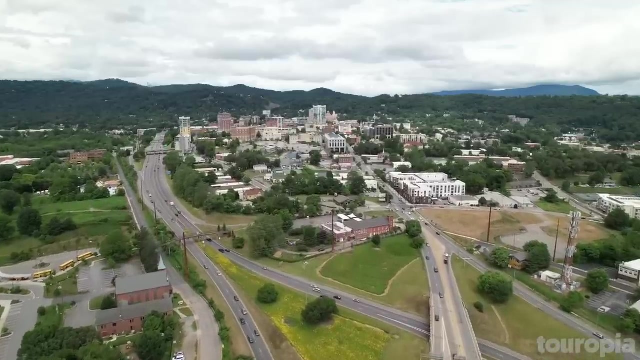 Visitors to Old Salem, for example, can watch shoemakers, gunsmiths and tailors go about performing their respective services or making their particular wares. Number 6. Asheville, Asheville- Asheville, The city of Asheville, which is set in the beautiful Blue Ridge foothills, enjoys a reputation. 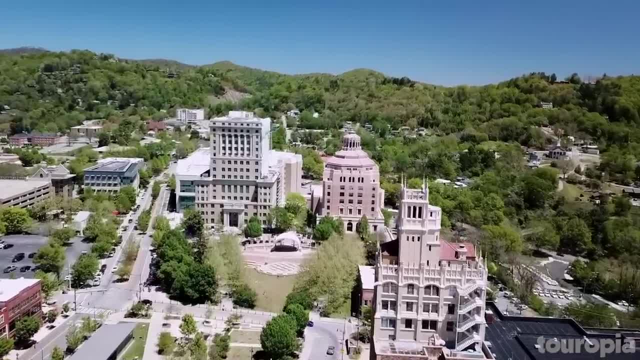 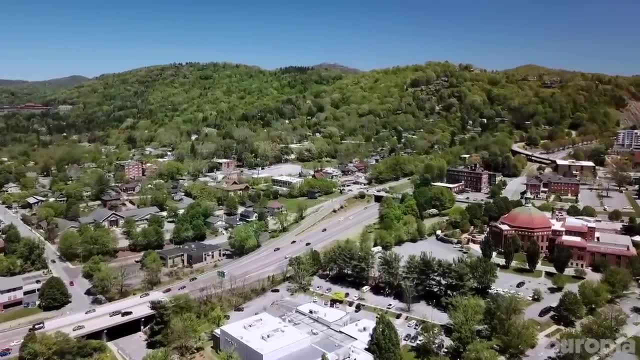 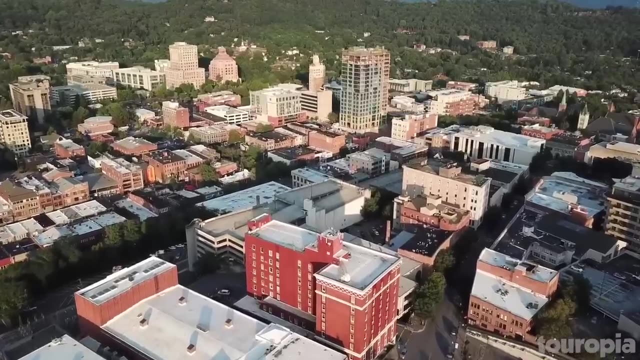 for being a vibrant artsy community. Its town center features a number of boutiques that showcase local creations, as well as bars and great places to eat. Strolling musicians and street performers only add to Asheville's overall creative vibe. The city is also located very close to the world-famous Biltmore Estate. 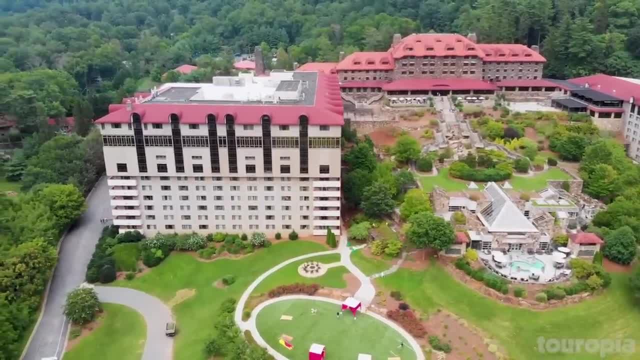 Built between 1889 and 1895,. this chateau-style estate was built in 1889 and 1891.. The Biltmore Estate was built between 1889 and 1895.. The Chateau-Styled Mansion is the largest privately owned house in the United States. 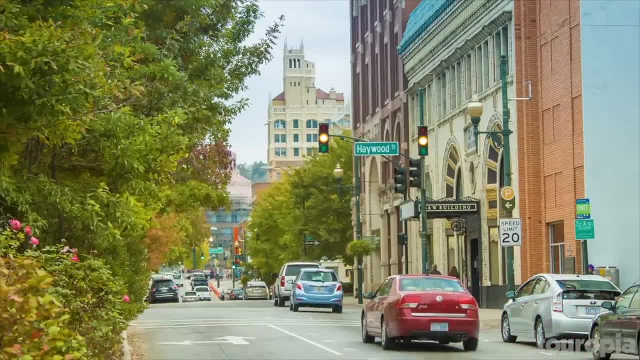 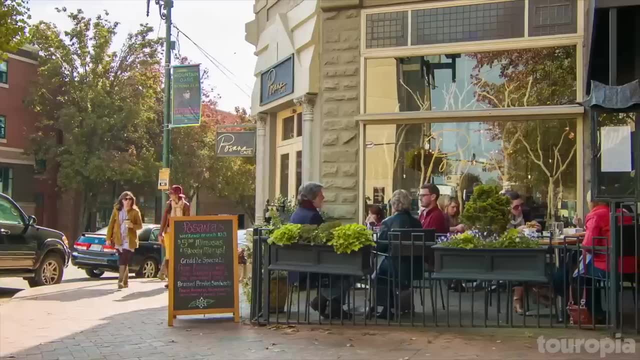 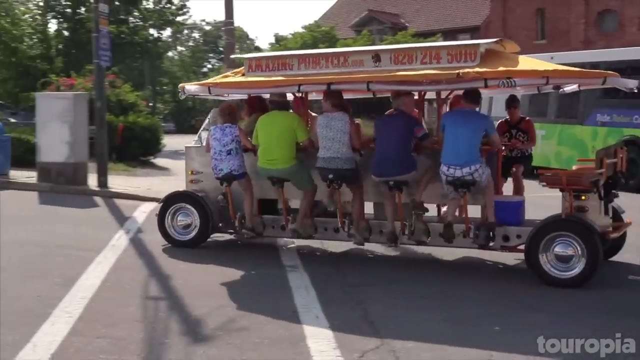 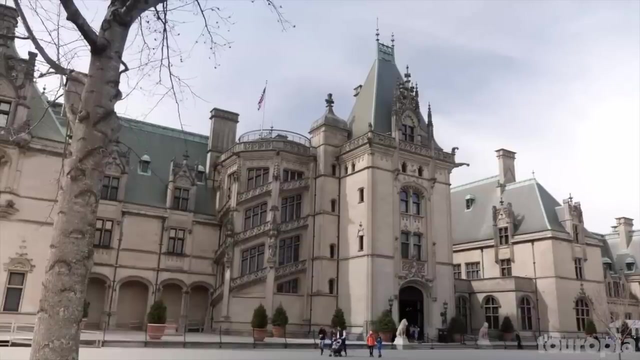 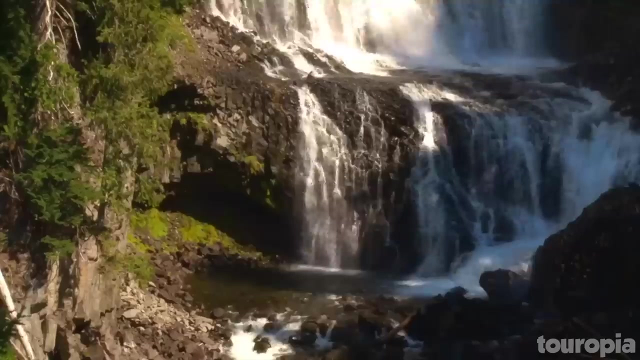 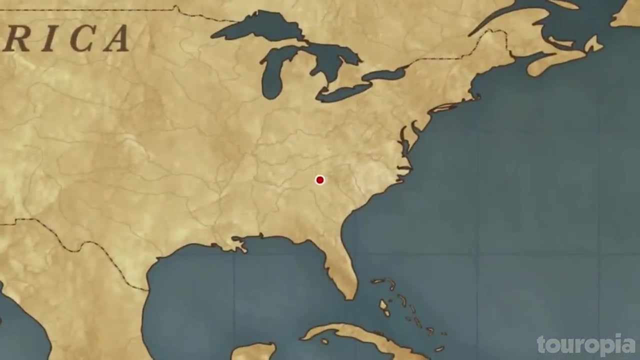 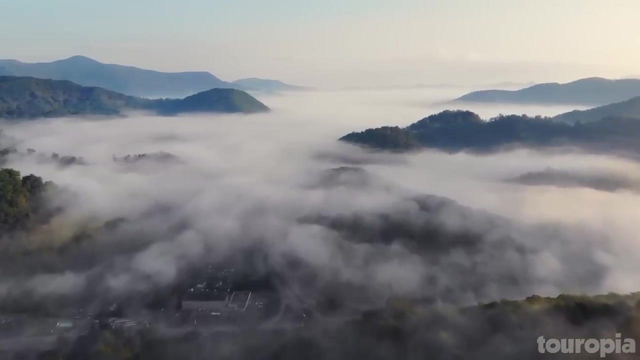 and attracts almost 1.5 million visitors each year. The Biltmore Estate was built in 1889 and 1891.. Number 5. Blue Ridge Parkway. The Blue Ridge Parkway is considered by many to be one of the most scenic roads in the. 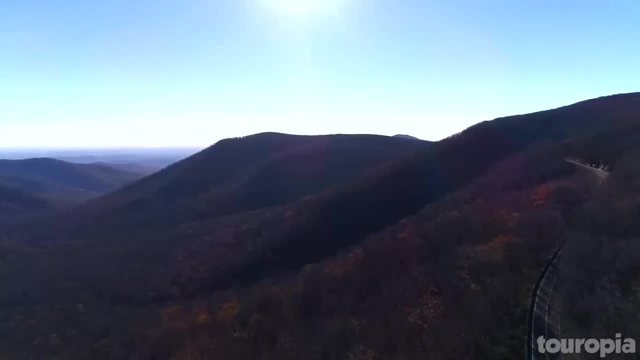 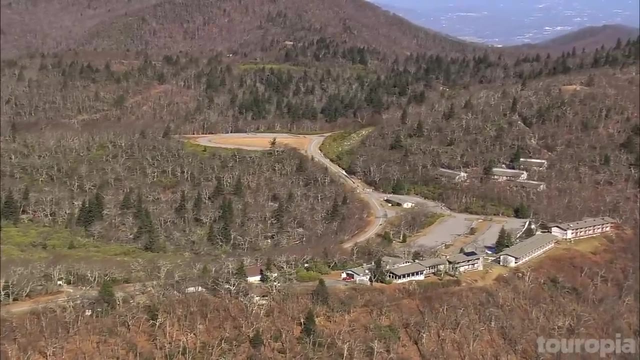 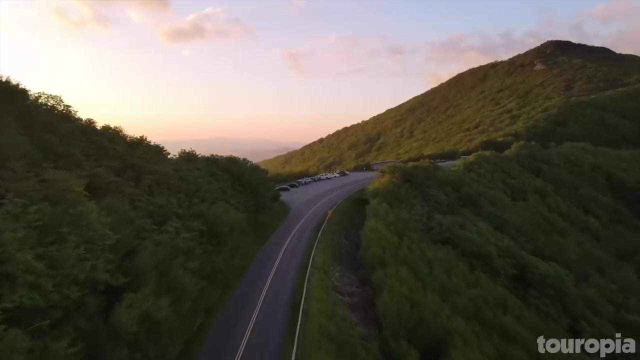 United States. It runs for 469 miles from the Great Smoky Mountains National Park to Virginia's Shenandoah National Park. This winding stretch of asphalt, which has earned both the National Parkway and All-American Road designations, is especially gorgeous during the fall months, when the surrounding 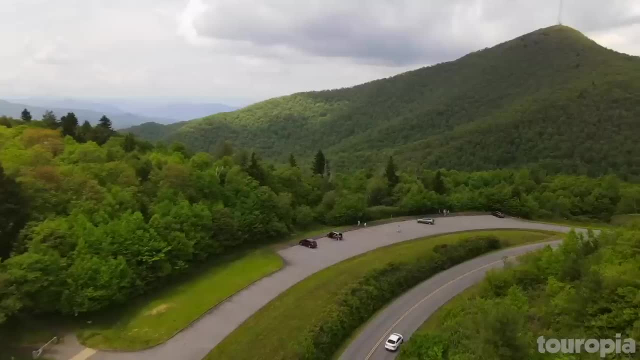 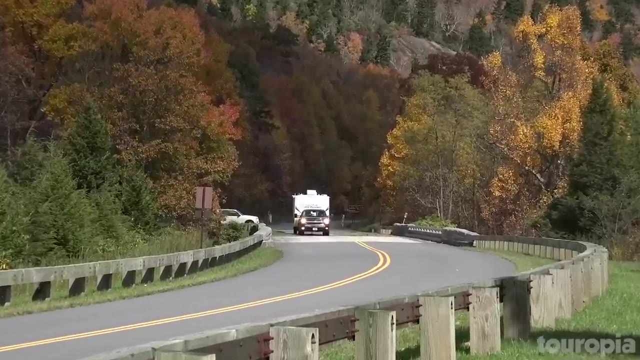 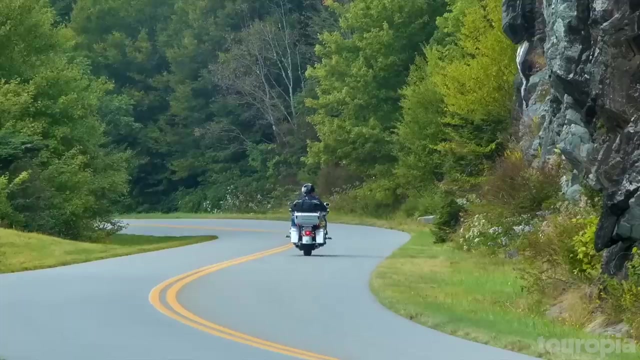 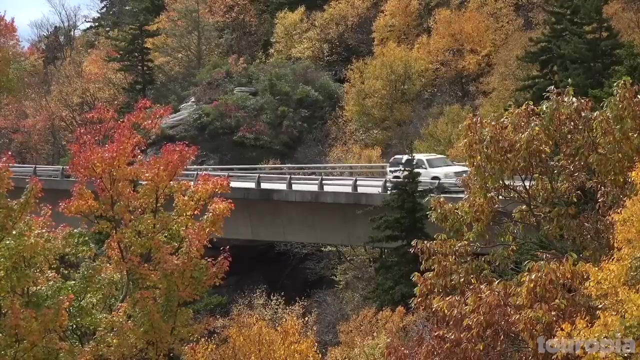 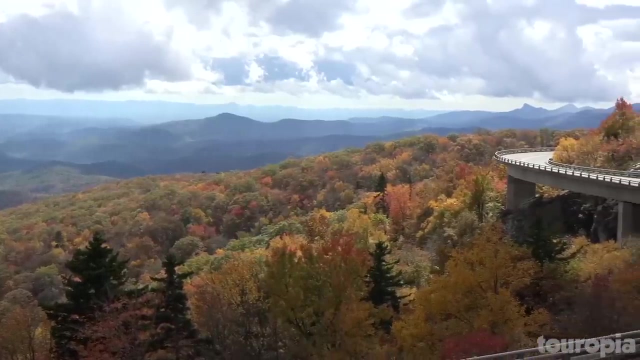 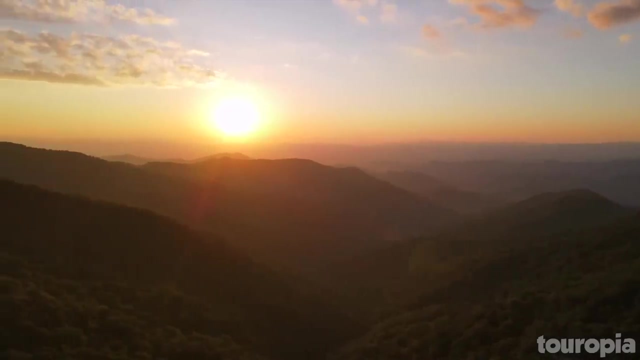 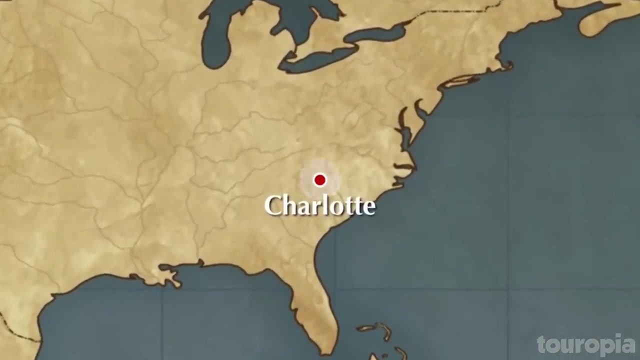 hills turn shades of oranges, yellows and reds. The parkway is also very pretty in the spring months when the Carolina rhododendrons and dogwoods are in bloom. Number 4. Charlotte, The largest city in North Carolina, Cosmopolitan Charlotte can be found in the southern part. 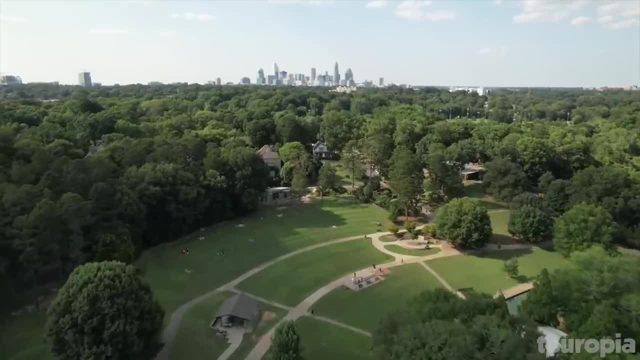 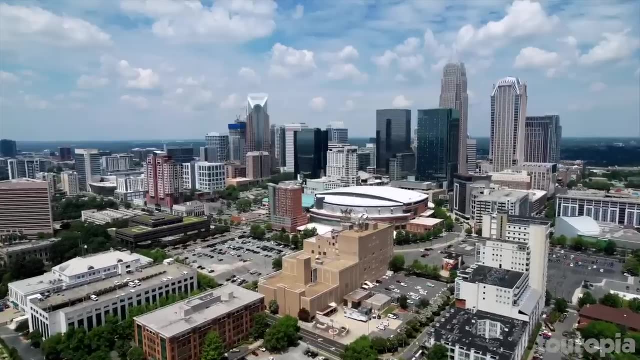 of the United States. It is the largest city in the United States. It is the largest city in the United States. It is found in the south center of the state, just a stone's throw away from South Carolina. It has a lot to offer visitors, especially those who love motorsports. 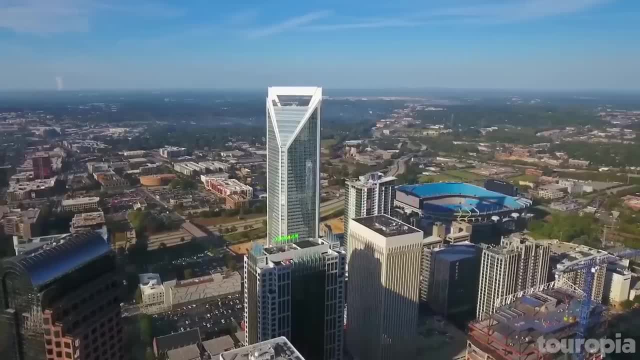 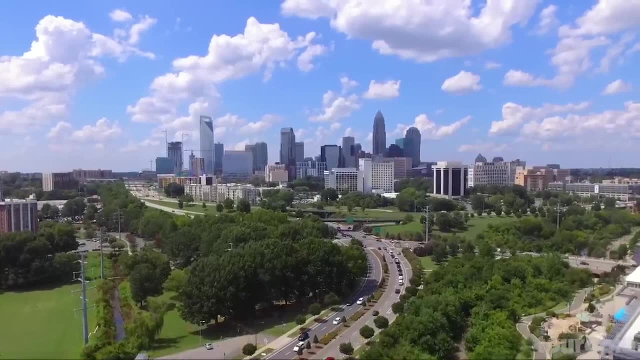 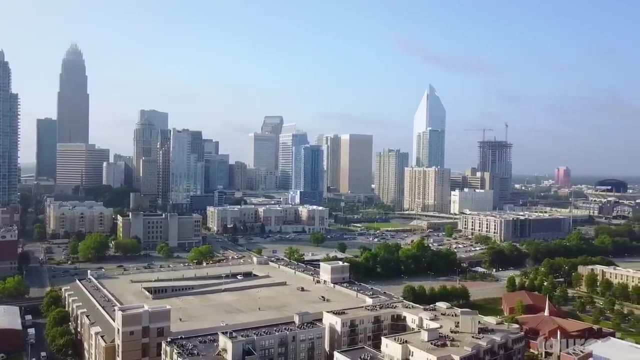 The Queen City is home to the Carowinds, the largest man-made whitewater park, the US National Whitewater Center and the family-friendly Discovery Place, which combines a science museum with an aquarium. This city is also where visitors can find the NASCAR Hall of Fame and Charlotte Motor. 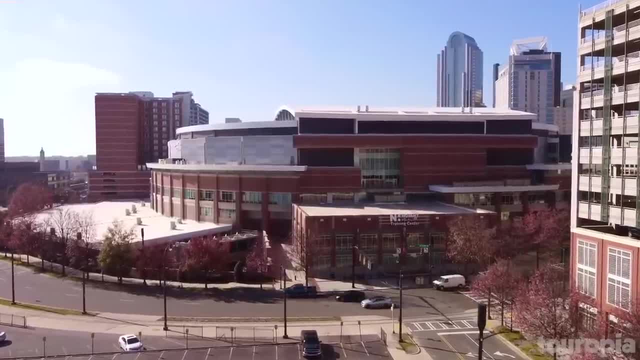 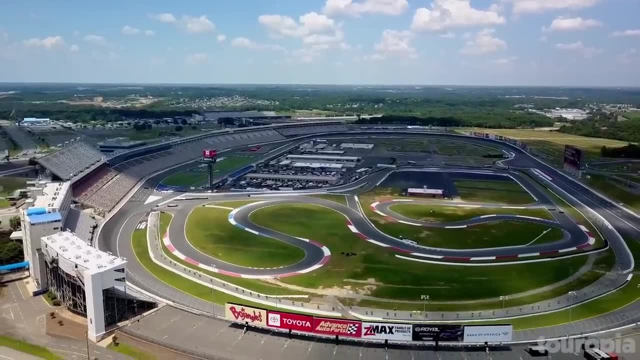 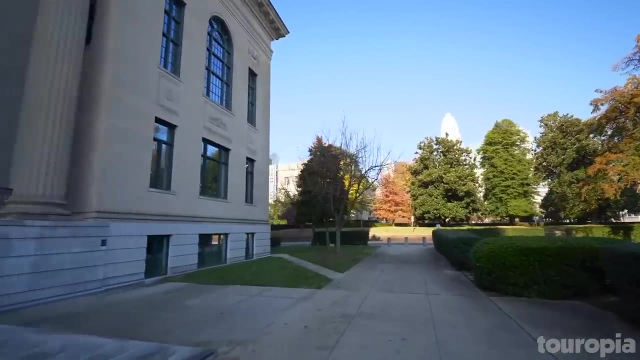 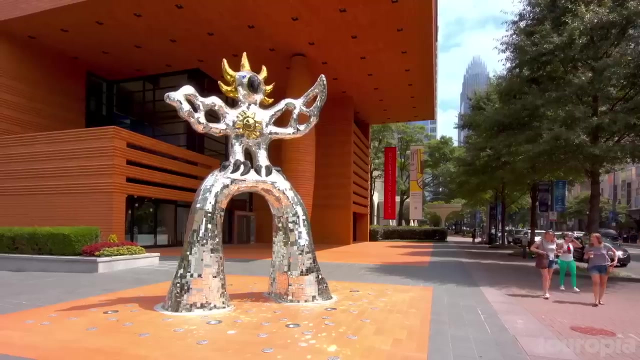 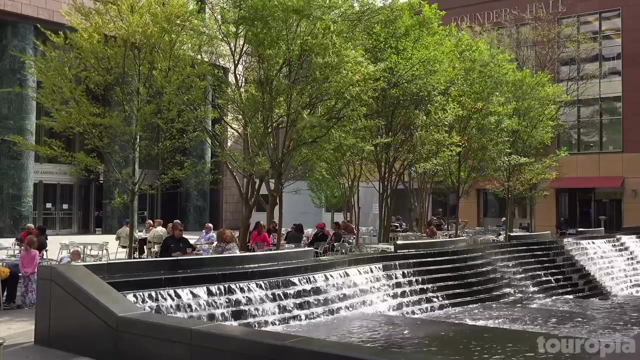 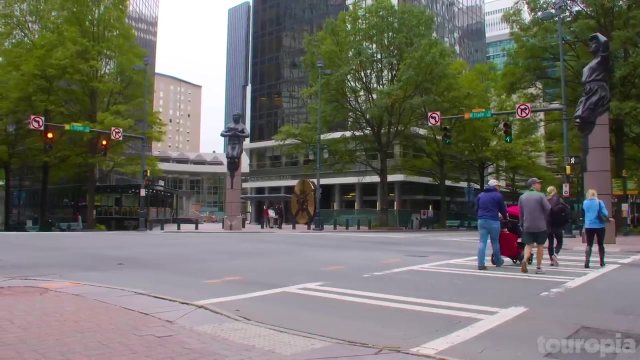 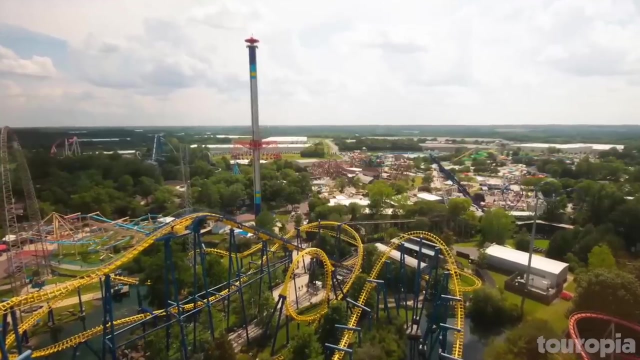 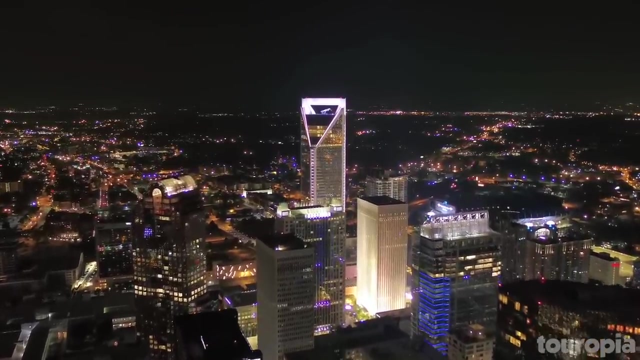 Speedway- Number 5.. Harry Potter and the Picasso rulebook. This week has won theSteve trucs statue of Harry Potter. It was named after sicilian emperor. Harry Potter, Number 6. Ne seria, Paris, Number 3.. Wilmington. The Wilmington area is home to some of North Carolina's most popular beaches: Carolina Cure and Wrightsville beaches. This historic port city is also a family-friendly destination. Its North Carolina Aquarium at Fort Fisher was named by the Travel Channel as one of 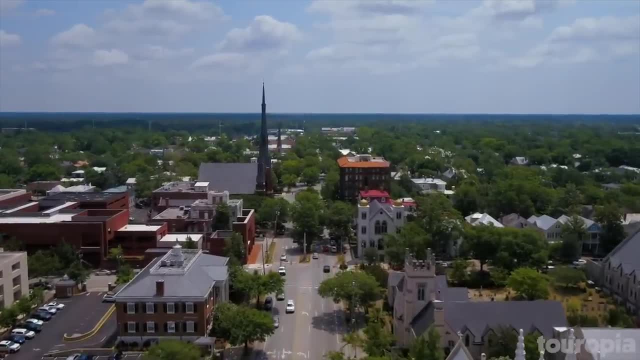 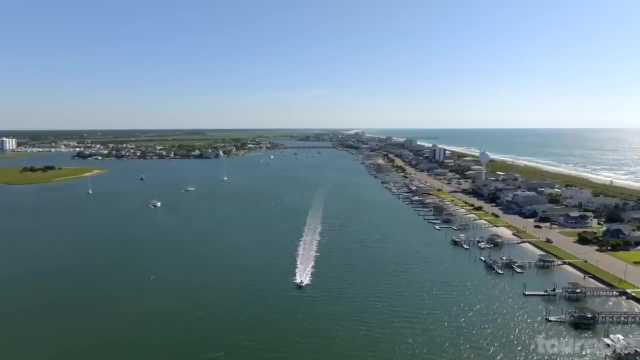 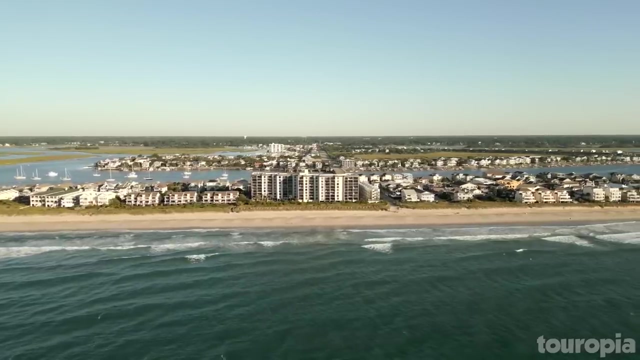 the best in the United States. Visitors can also enjoy taking leisurely strolls along Wilmington's Riverwalk, which runs alongside the Cape Fear River. There are a number of mansions and plantations in the area, including Poplar Grove Plantation, the oldest peanut plantation in the United States, and the 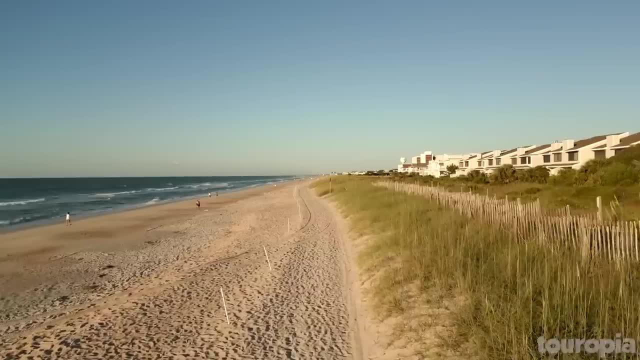 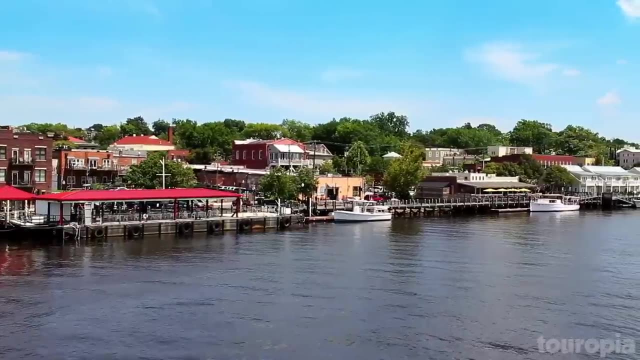 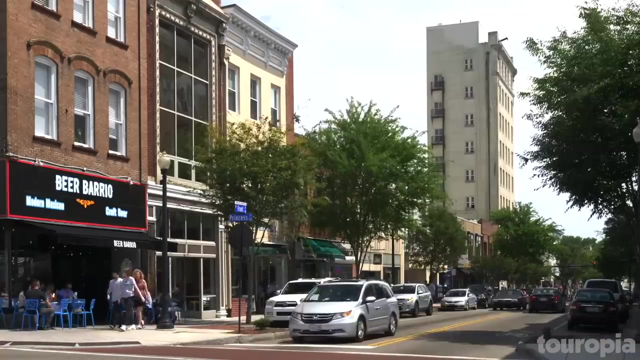 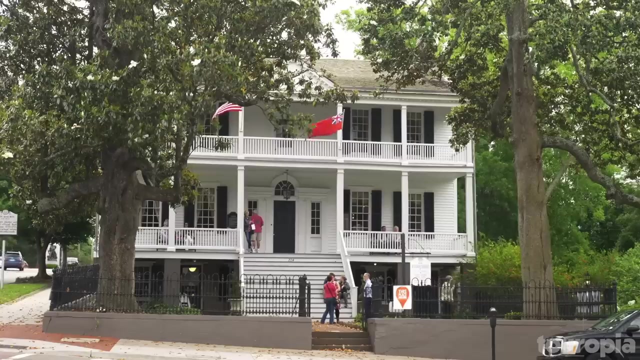 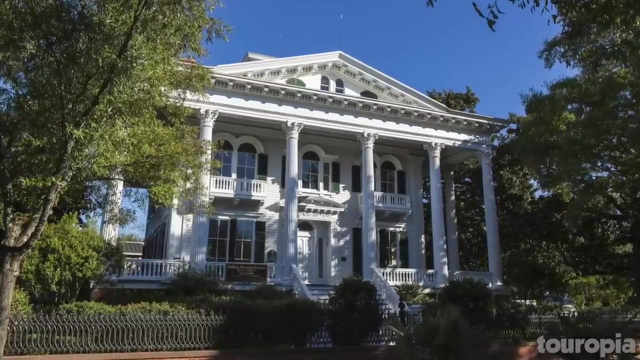 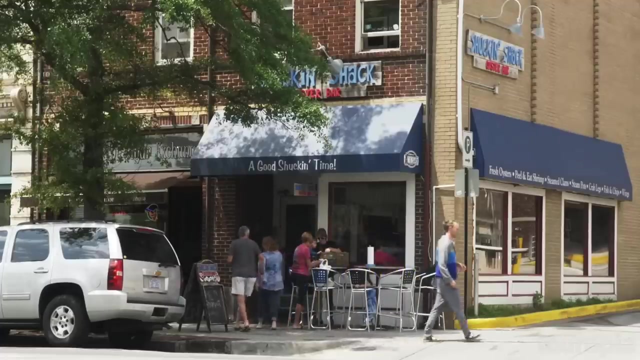 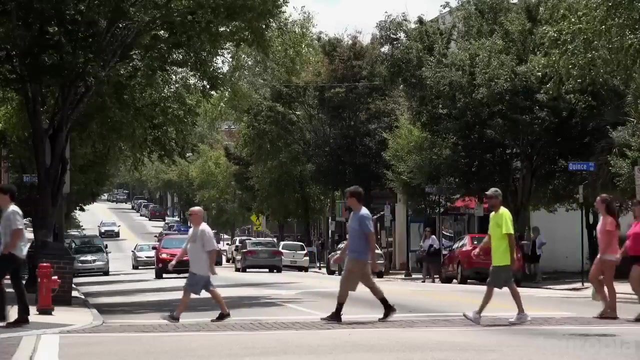 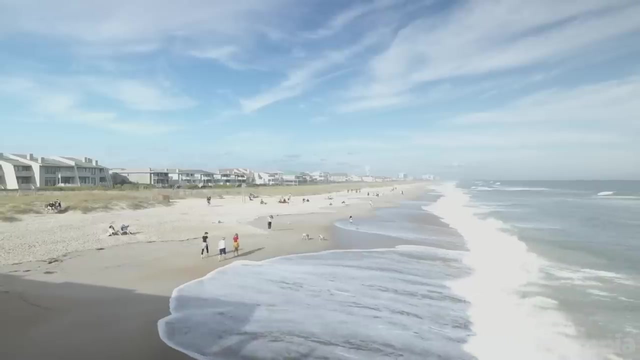 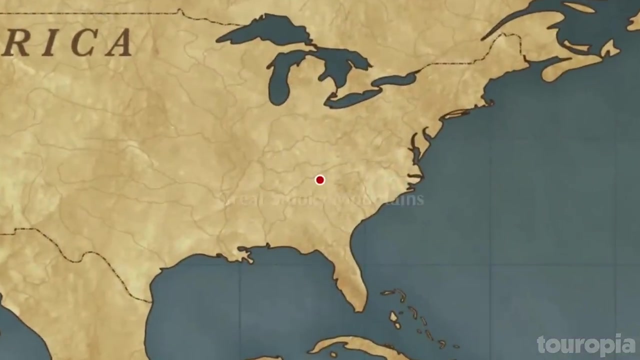 antebellum Bellamy Mansion. There are a number of ort 예�ores and prima l bu set ylene расс ٩ tan degradation o l en gla. architecture Number 2. Great Smoky Mountains: This national park is a world of beautiful nature. 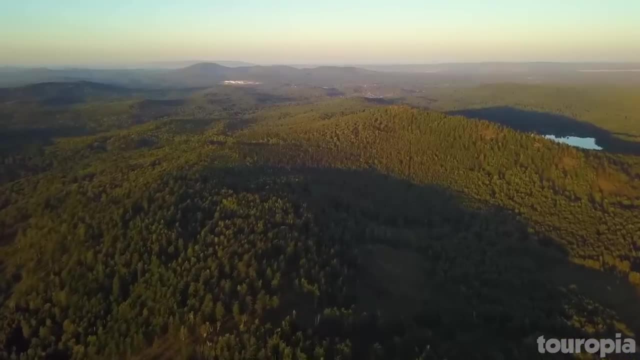 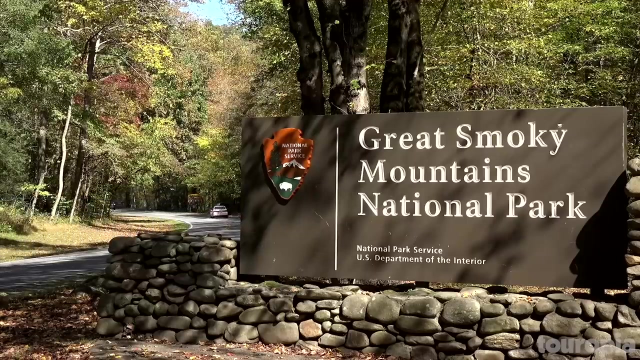 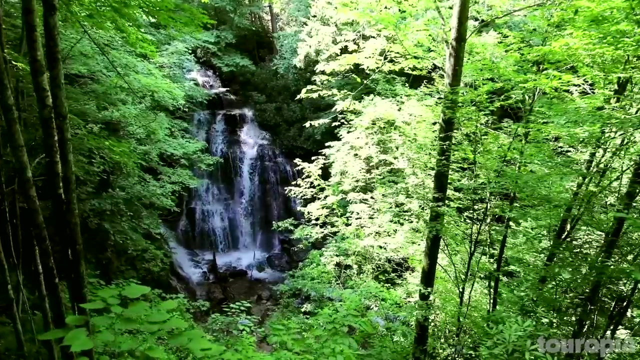 Think verdant forests as far as the eye can see, glistening waterfalls and undulating mountain peaks. The forests themselves come alive in springtime, with a rainbow of wildflowers blazing between the trees, Autumn brings the famous fall foliage for a sea of auburn, and winter is all about snow. 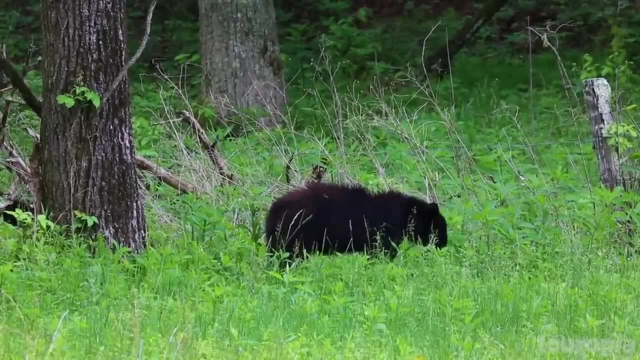 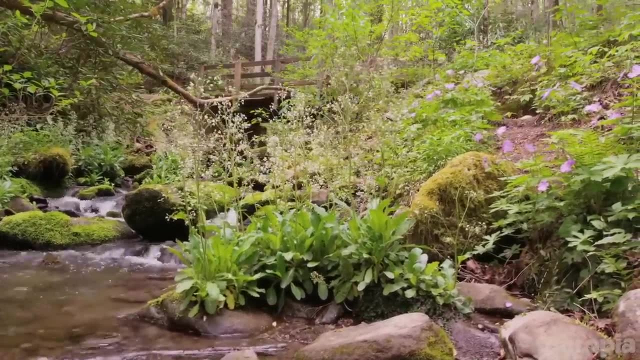 Dubbed the Smokies because of the misty mountaintops. exploring this national park is like stepping into the past. There are still remote mountain communities who call this region home. It's a great spot to truly unwind and leave the modern world behind. Number 1. Outer Banks. The Outer Banks is a string of barrier islands that hug the North Carolina coastline. The islands are a popular tourist destination. The islands are a popular tourist destination. The islands are a popular tourist destination. It's a popular destination for vacationers seeking a break from the summer heat. The northern end of the Outer Banks is famous for the wild horses that still wander its dunes. The middle section is home to the towns of Nags Head and Kitty Hawk on Bodie Island, where travelers can find the Wright Brothers National Memorial. Roanoke Island, west of Bodie Island, was once home to the Lost Colony, whose inhabitants disappeared without a trace in the 1580s. Farther south lies the beautiful and relatively wild Cape Hatteras National Seashore. From this beautiful view you can follow the wild horses that, in most of their lives, have left a mark on our history. Look for them at the outers banks on the west bank, the river and the waterfront. The outers banks are home to a unique group of hunters. There are numerous animals to be found, including raccoonsmen and blockchain. This line is one of the most beautiful and rare species of creatures in the world. To see how the wild horses can be found, visit our website, http//wwwhatterasorg. Outer Banks is home to the notable wild horses and all the local people's. 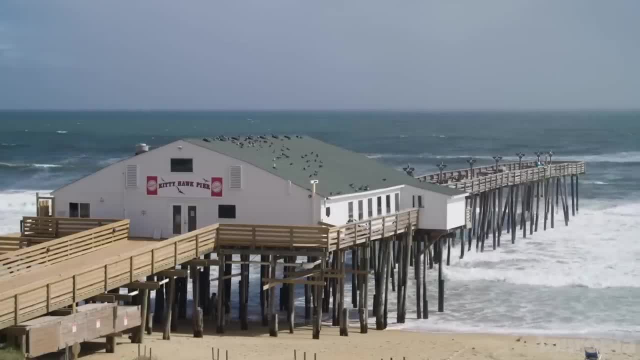 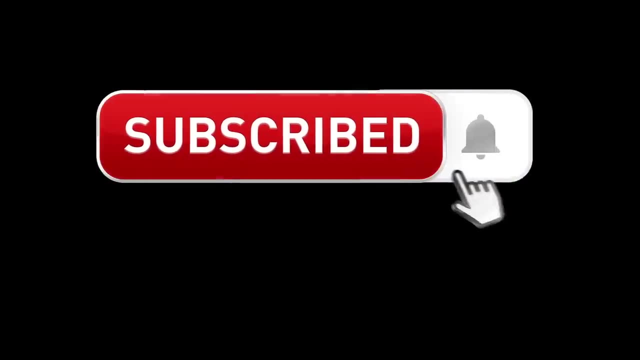 lidt Outer Banks is home to the wild horses and all the local people's anxieties. Thank you for watching.